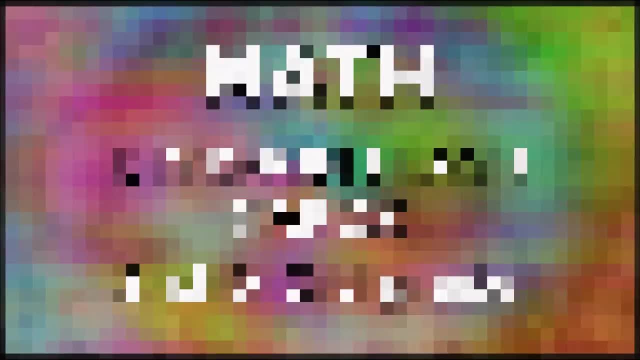 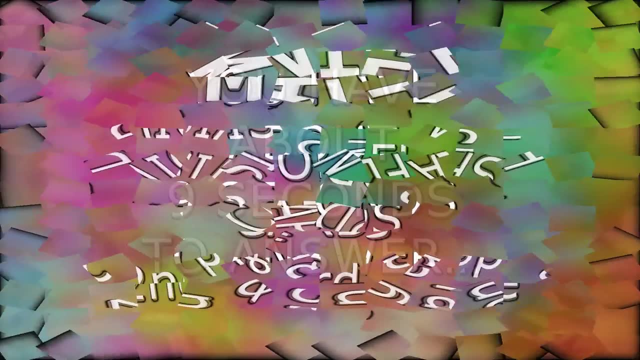 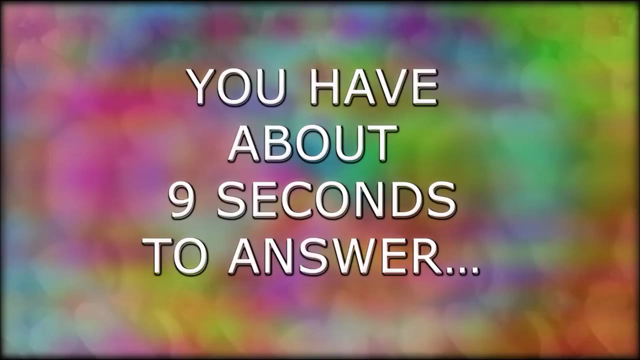 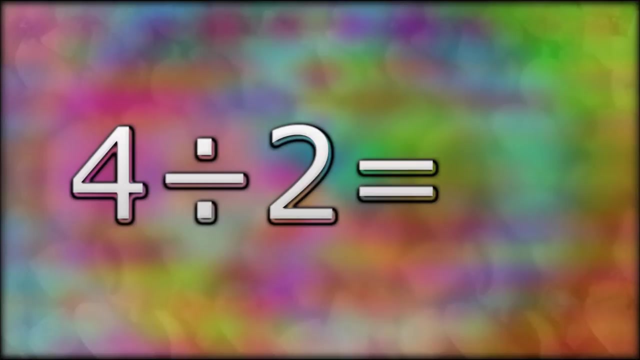 Math Division flashcards- 2nd and 3rd grade. You have about 9 seconds to answer. 4 divided by 2 equals 2.. 5 divided by 1 equals 5.. 8 divided by 2 equals. 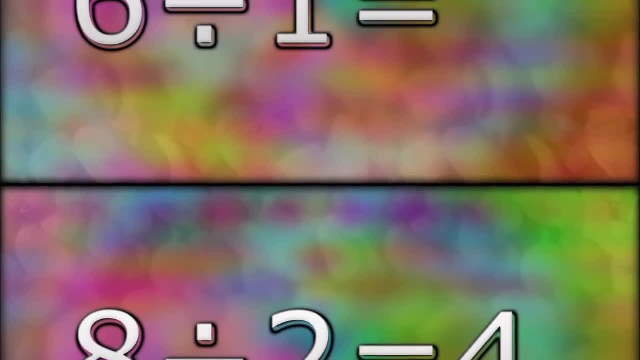 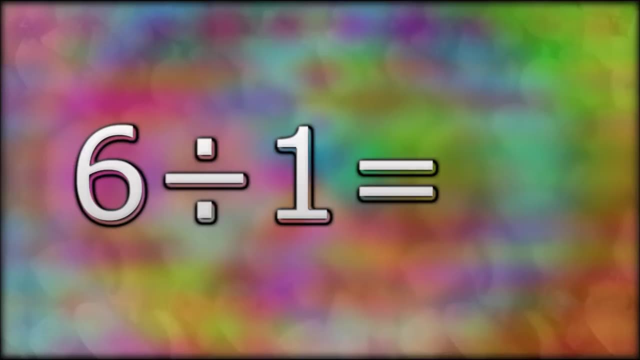 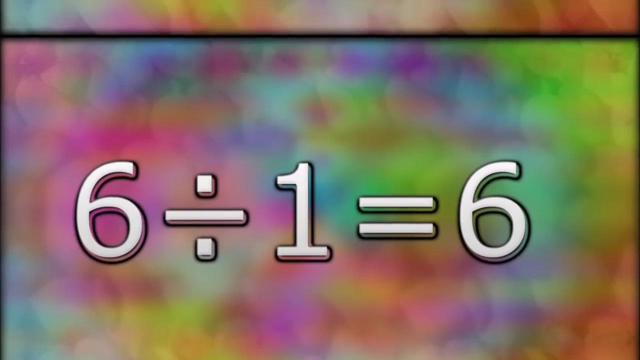 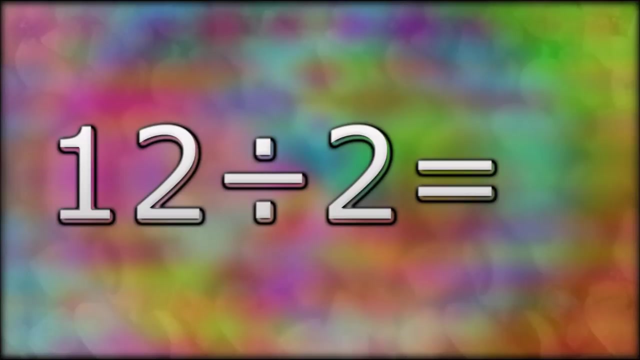 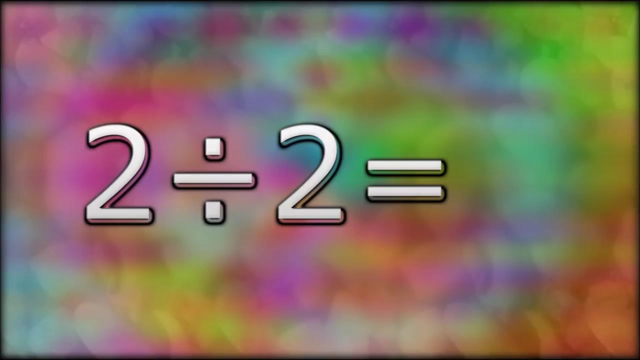 4. 6 divided by 1: equals. 6. 12 divided by 2: equals. 6. 2 divided by 2: equals. 6. 2 divided by 2: equals. 6. 1. 8 divided by 1: equals. 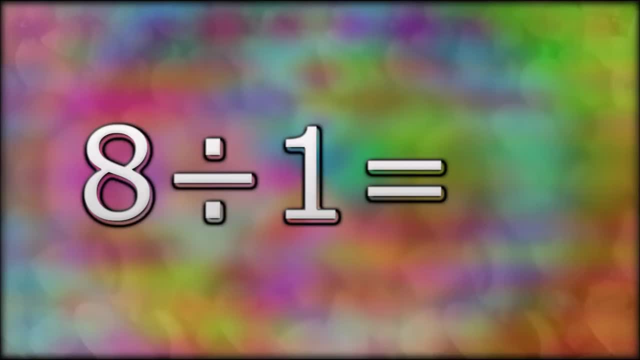 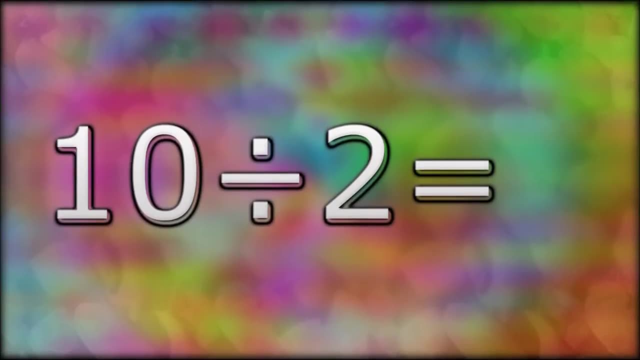 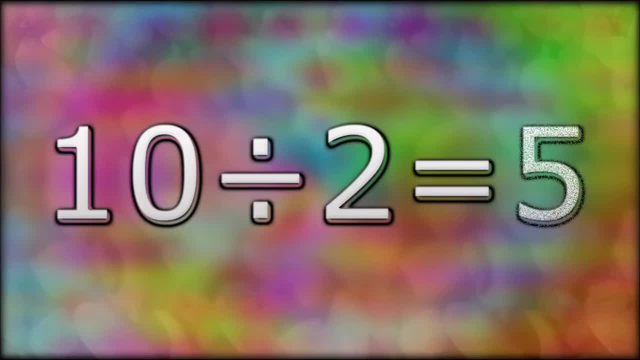 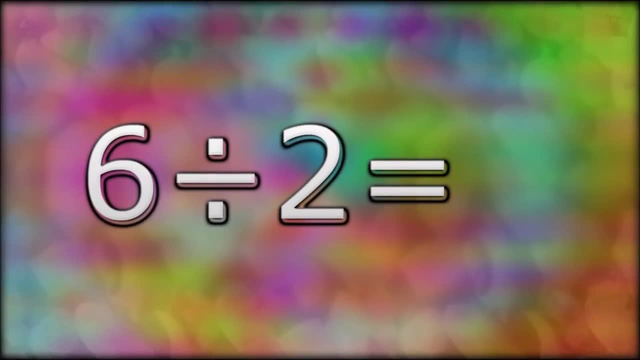 8. 8. 8 divided by 1 equals 8. 8. 8 divided by 1 equals: 8. 8 divided by 1 equals 8. 8. 8 divided by 1 equals. 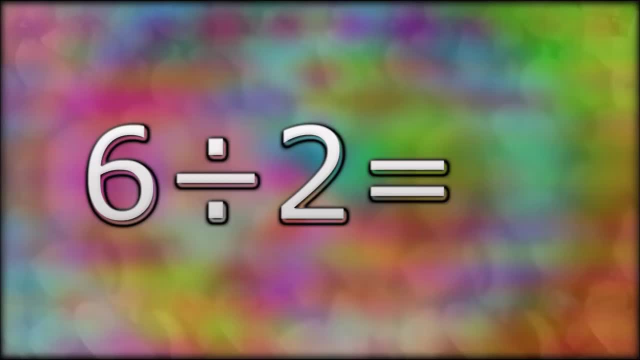 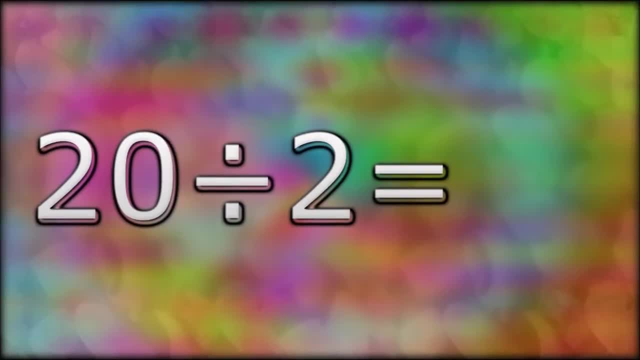 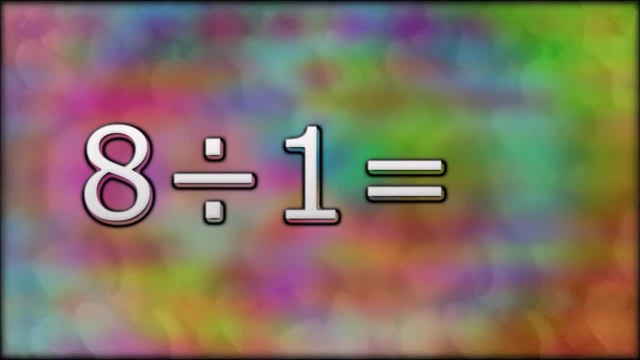 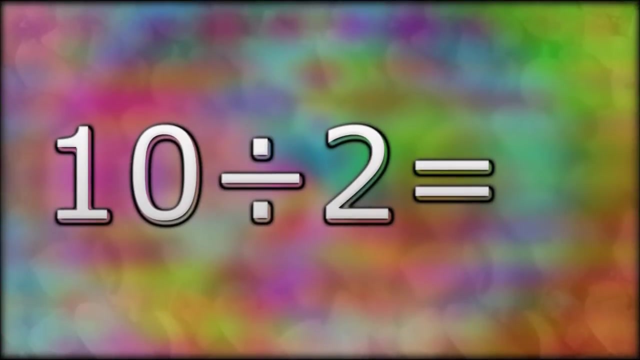 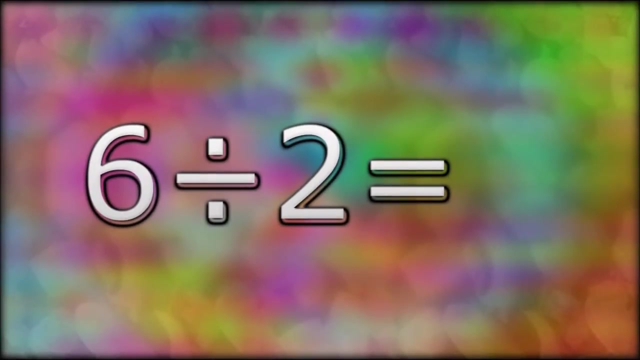 6.. 2 divided by 2: equals 6.. 2 divided by 2: equals 6.. 2 divided by 2 equals 6.. 10 divided by 2 equals 5. 6 divided by 2 equals 3. 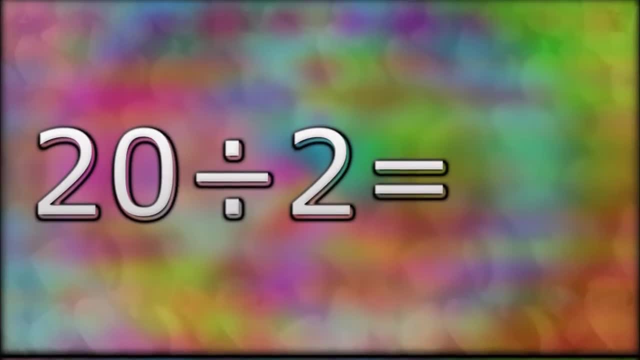 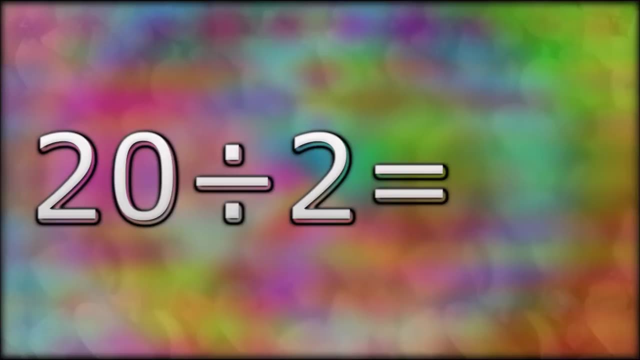 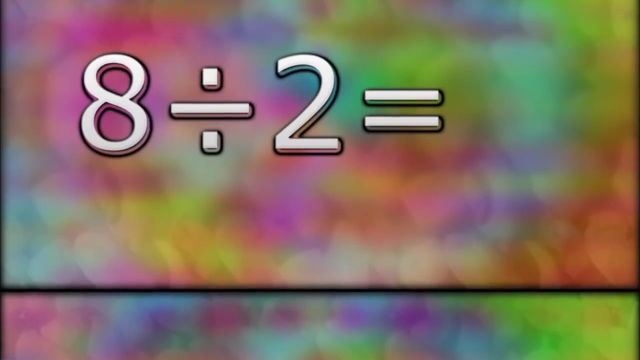 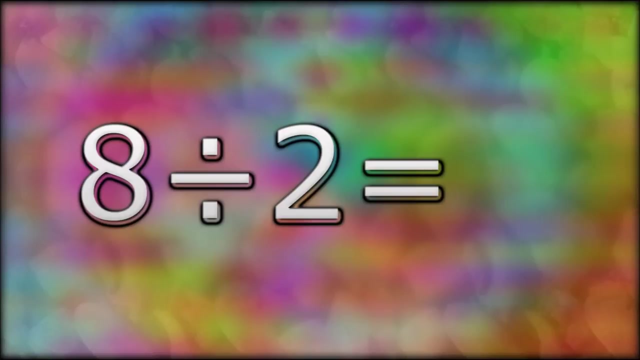 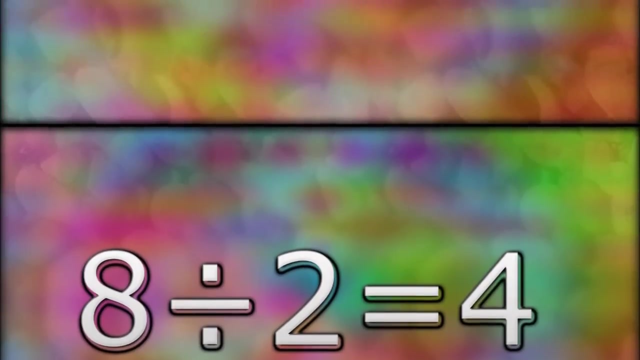 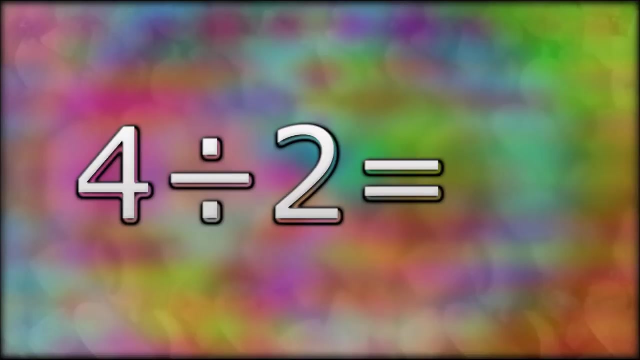 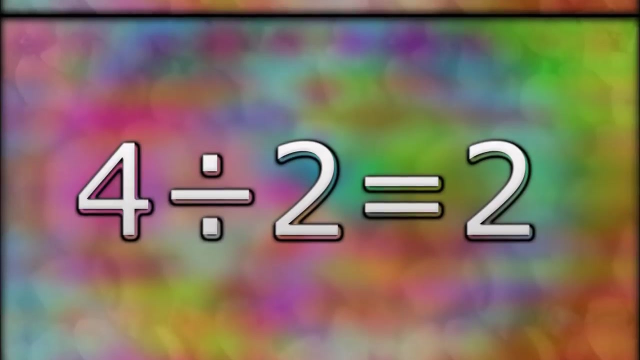 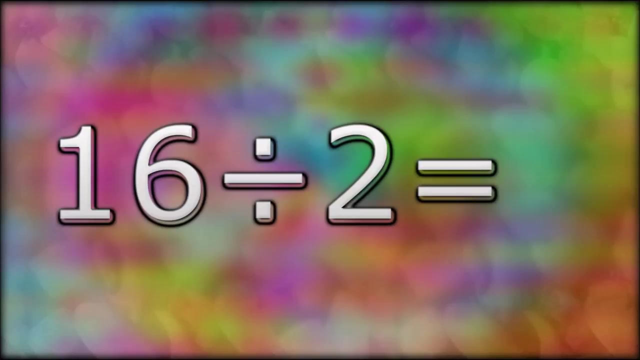 20 divided by 2 equals: 10, 8 divided by 2 equals. 4. 7 divided by 2 equals: 3, 4 divided by 2 equals: 2, 16 divided by 2 equals. 8. 6 divided by 2 equals. 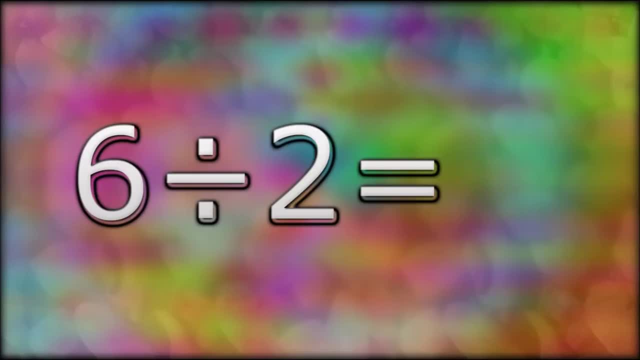 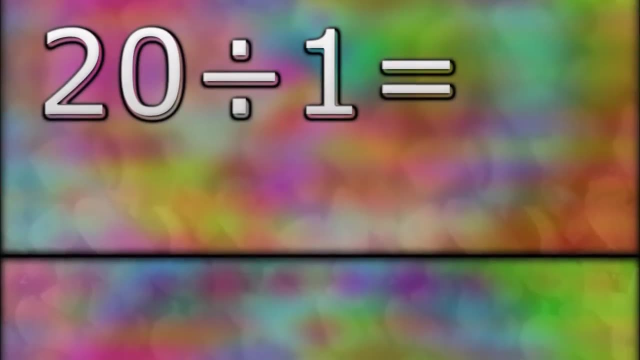 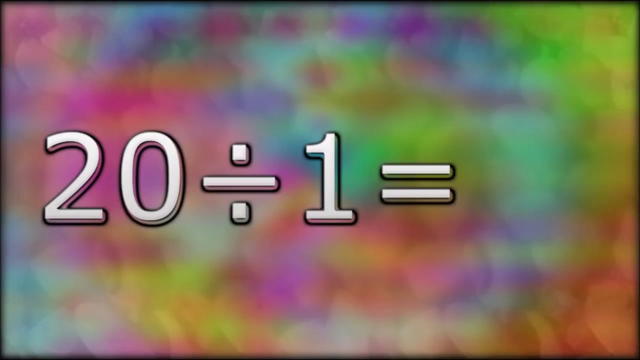 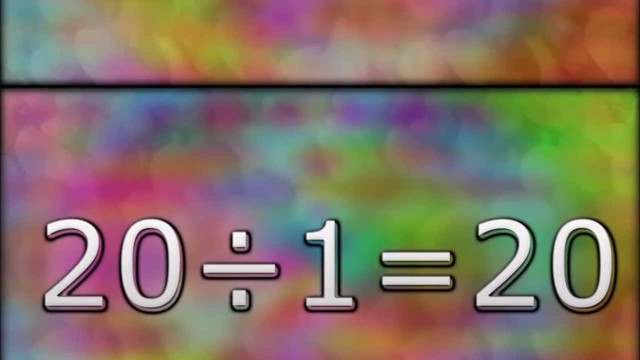 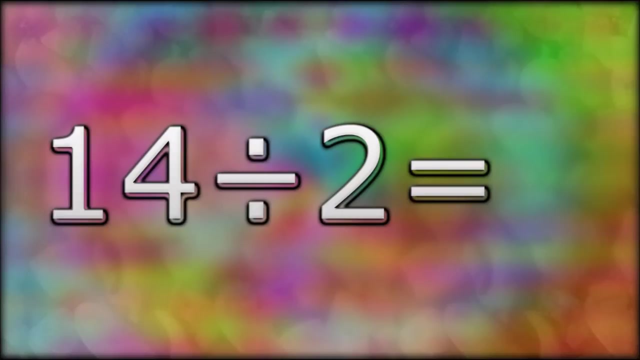 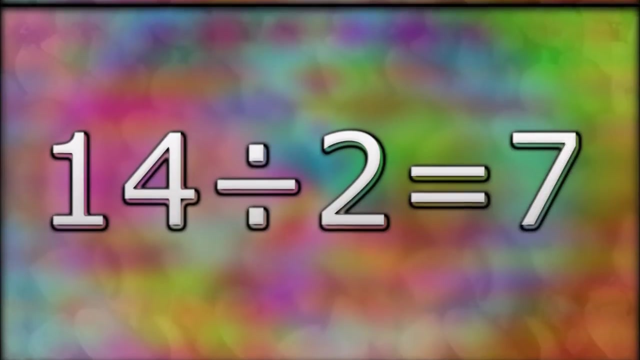 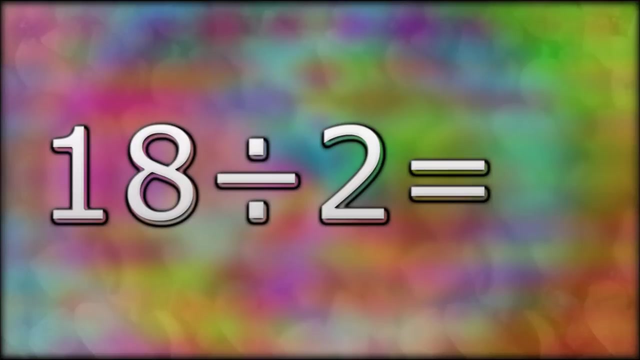 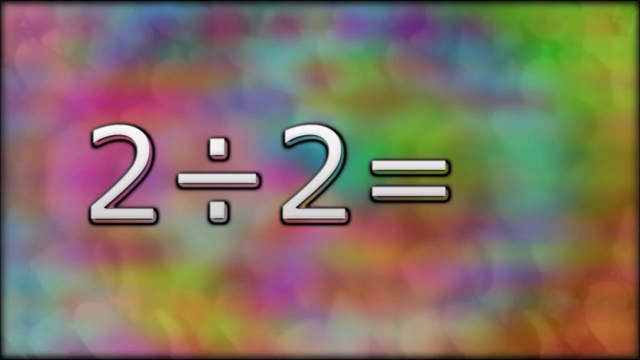 3, 20 divided by 2 equals. 4 divided by 1 equals 20, 14 divided by 2 equals 7, 18 divided by 2 equals. 9, 2 divided by 2 equals. 1, 24 divided by 2 equals. 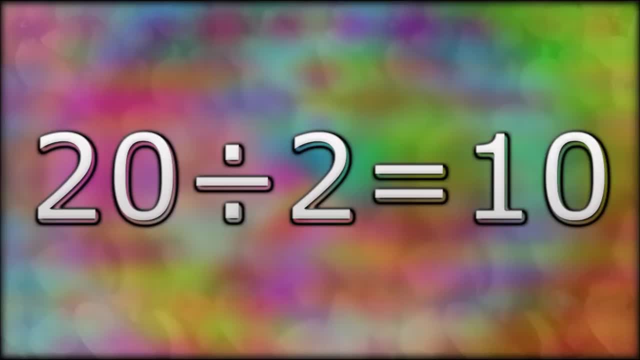 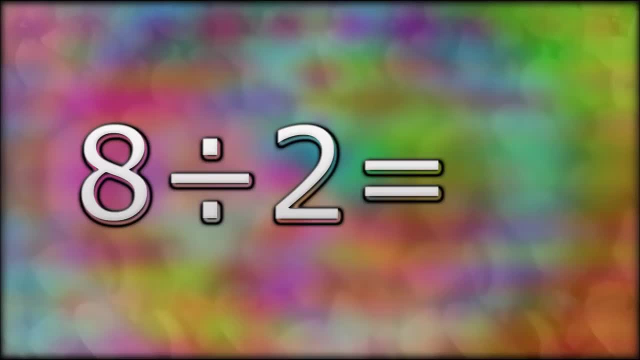 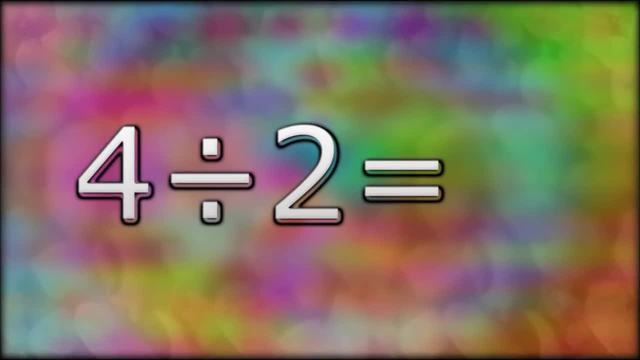 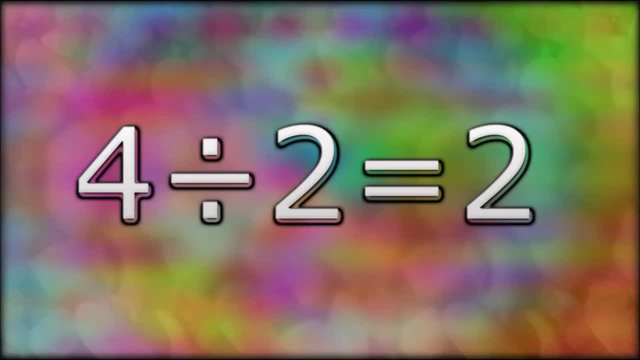 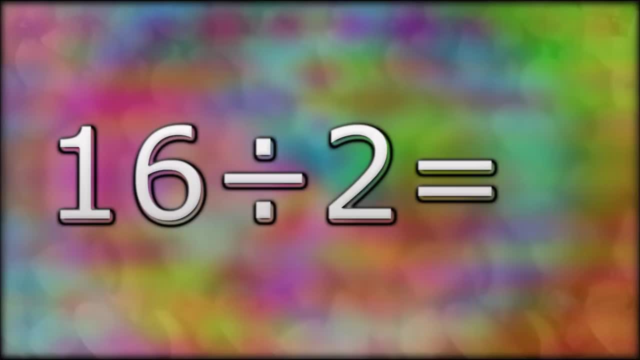 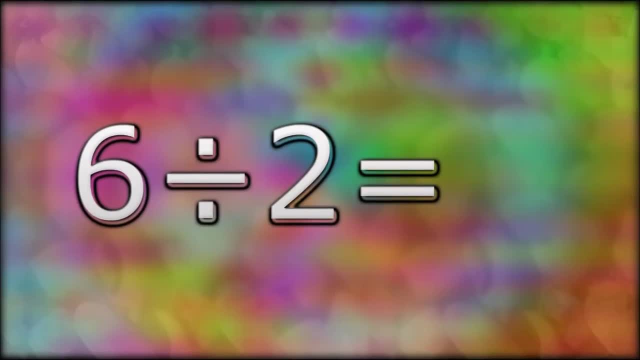 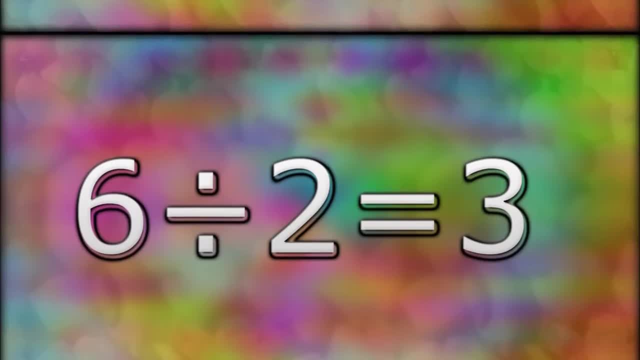 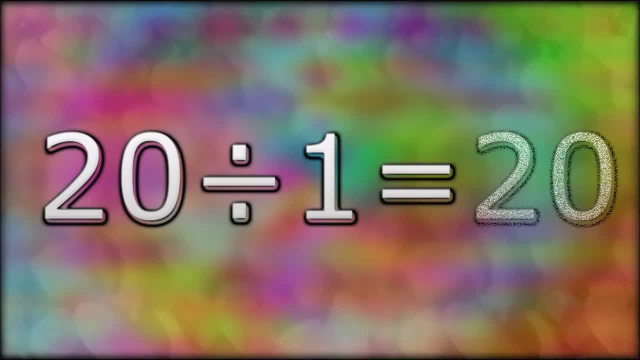 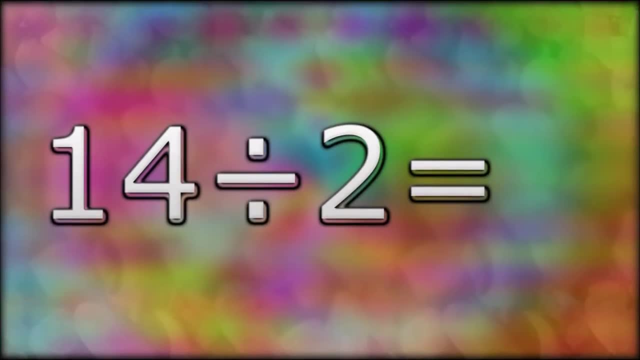 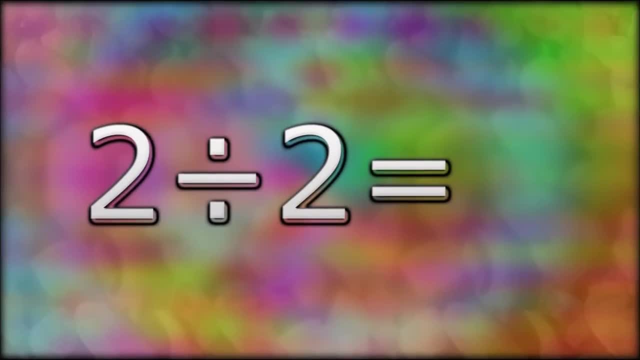 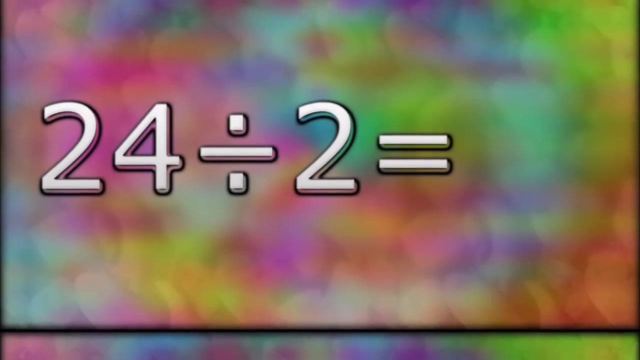 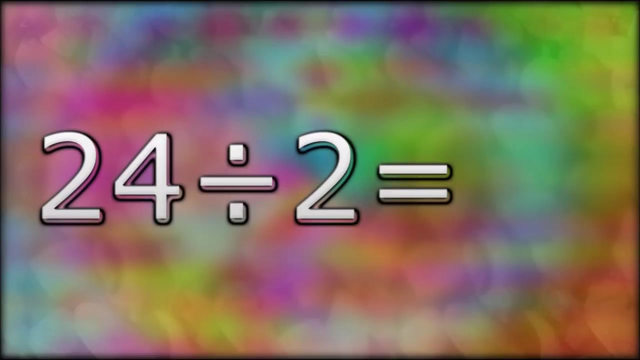 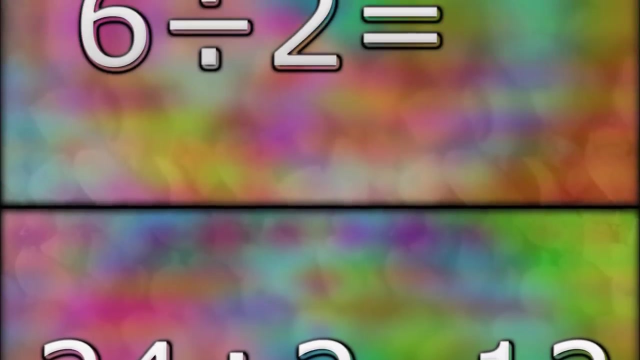 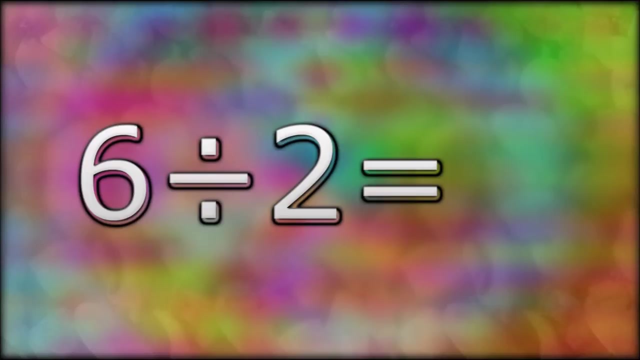 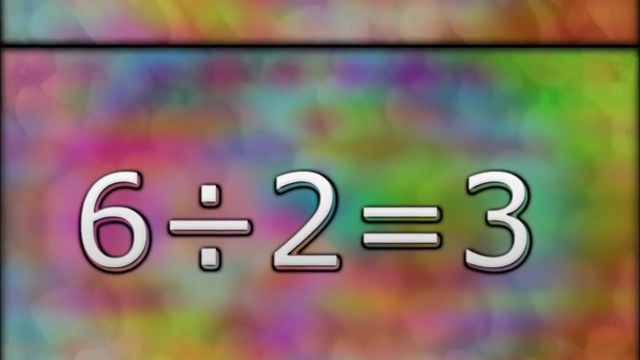 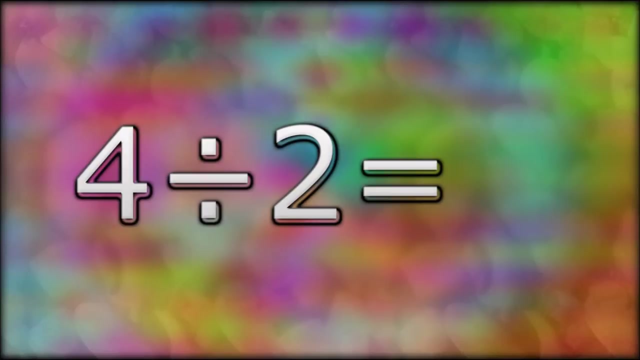 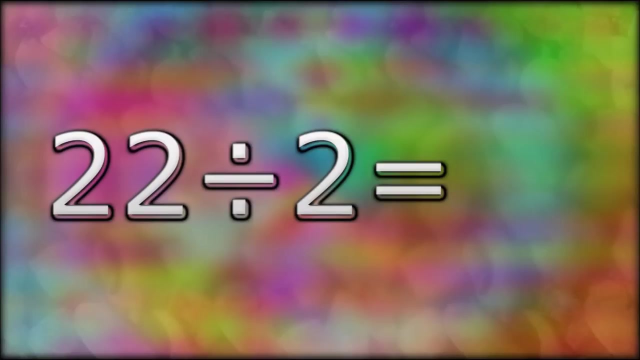 2 divided by 2 equals 1. 24 divided by 2 equals 12. 14 divided by 2 equals 6 divided by 2 equals 3. 4 divided by 2 equals 2. 22 divided by 2 equals 11. 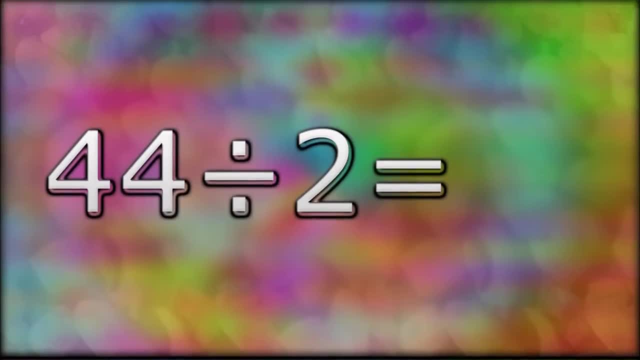 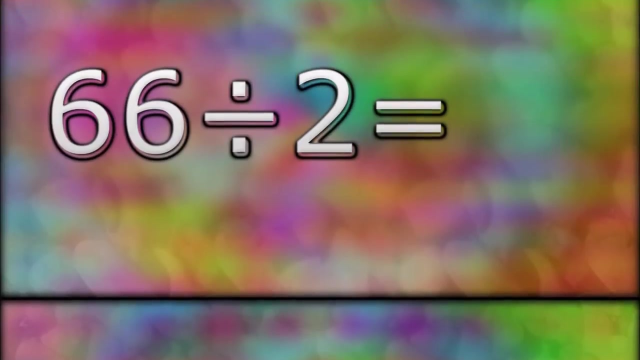 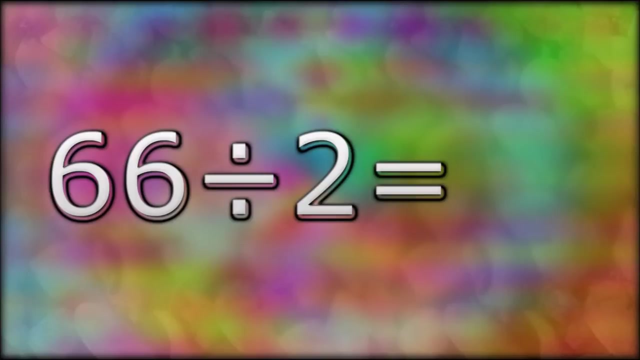 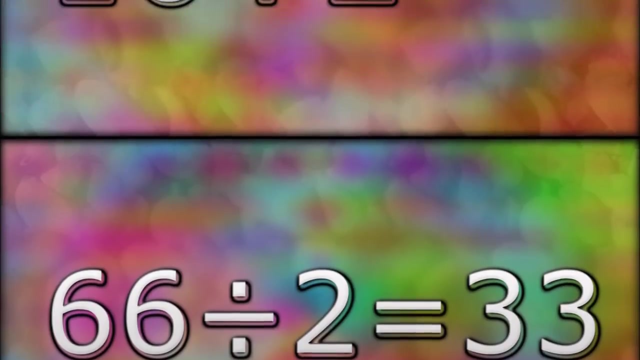 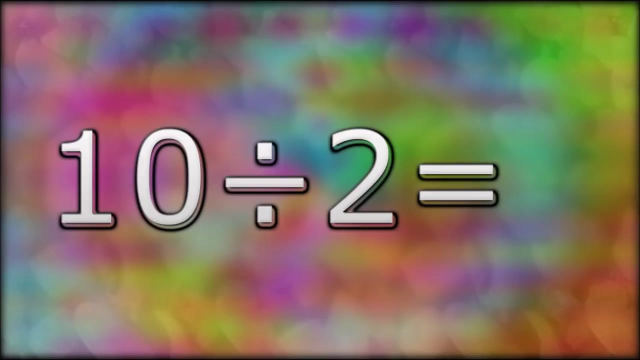 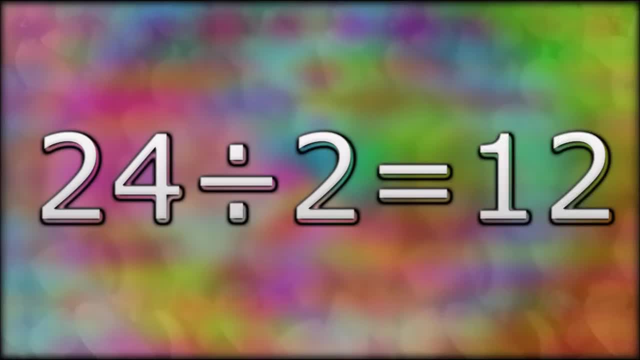 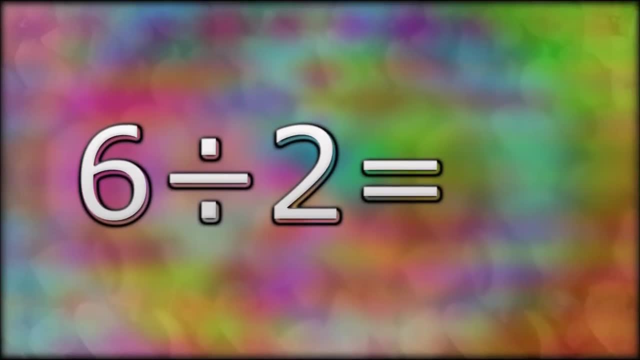 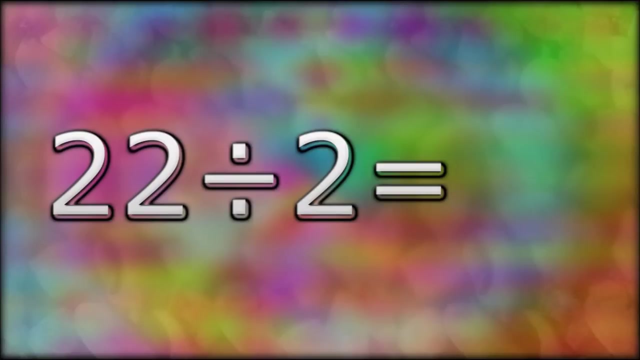 12: 12, 6 divided by 2 equals. 3, 4 divided by 2 equals. 2, 7 divided by 2 equals. 8, 2 divided by 2 equals. 3, 2 divided by 2 equals. 3, 2 divided by 2 equals. 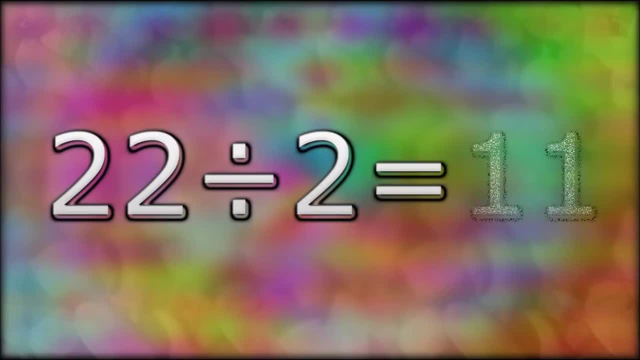 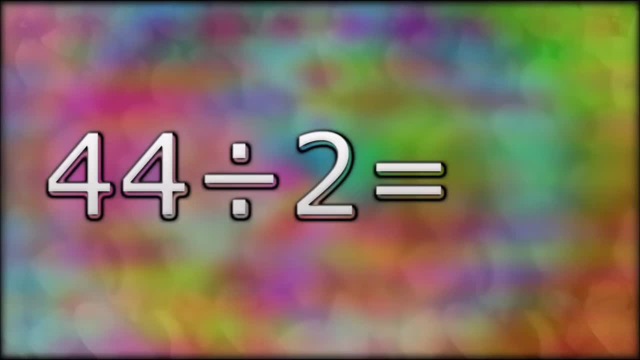 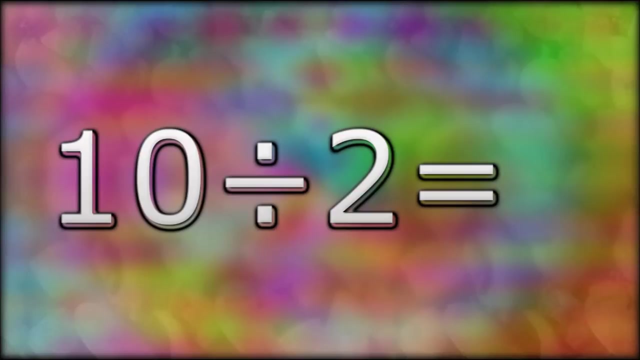 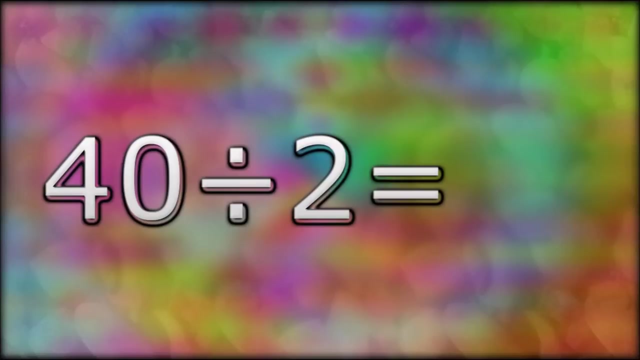 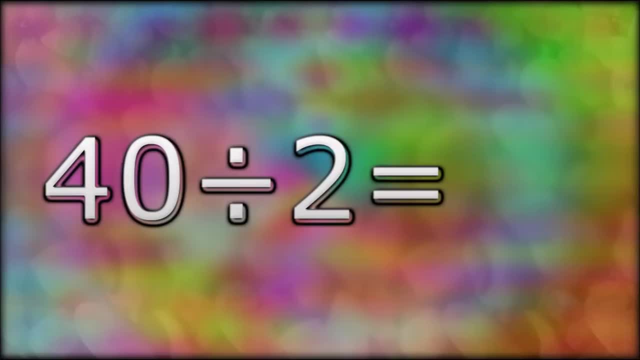 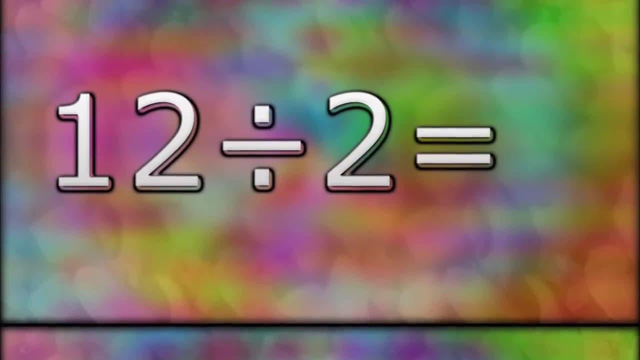 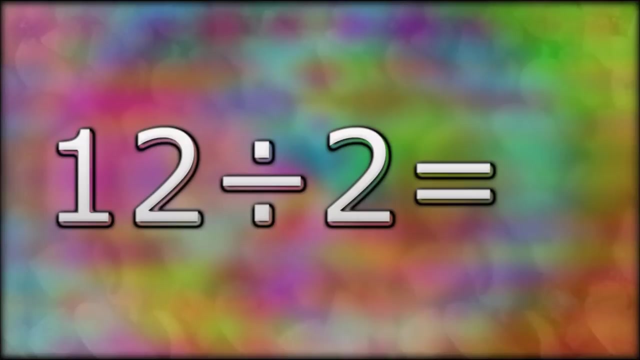 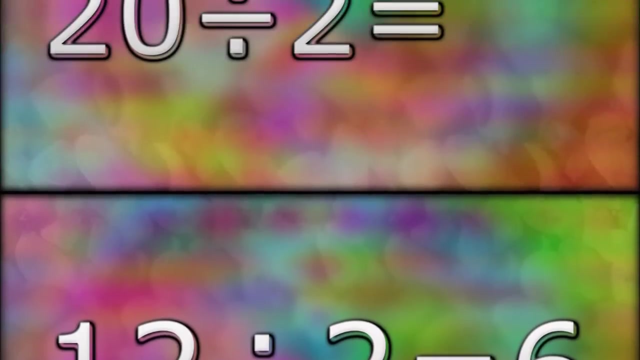 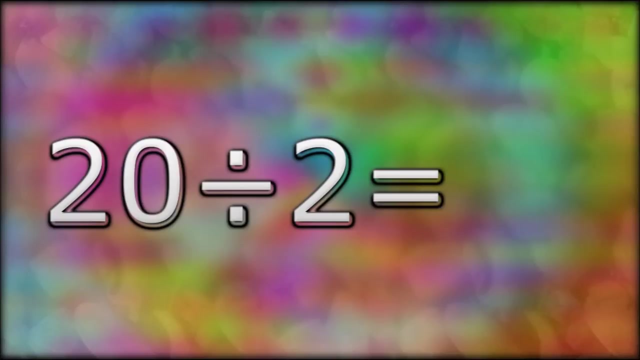 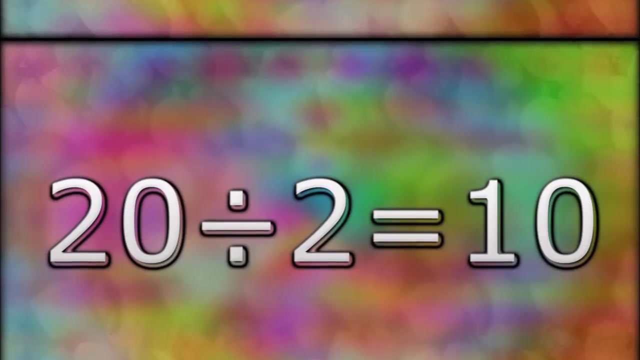 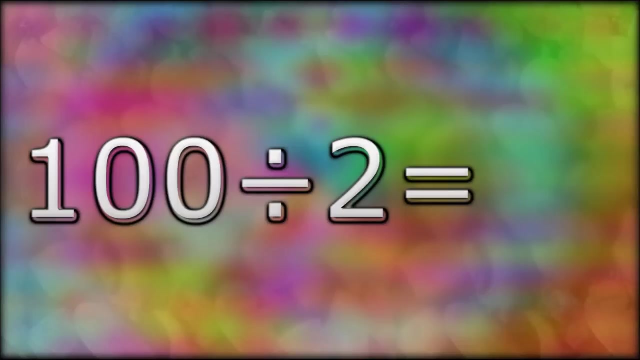 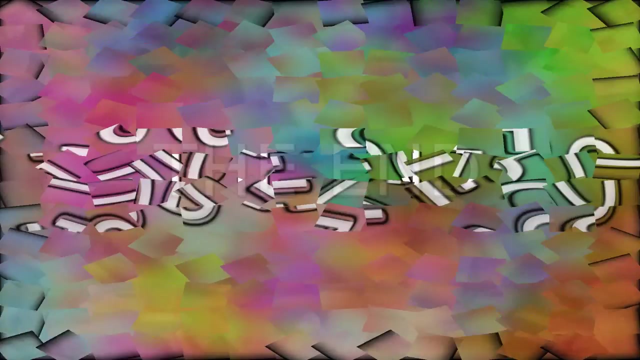 Ten, Twenty Twelve divided by two equals Six. Twenty divided by two equals Eight. Twenty-three 100 divided by 2 equals 50.. The end.